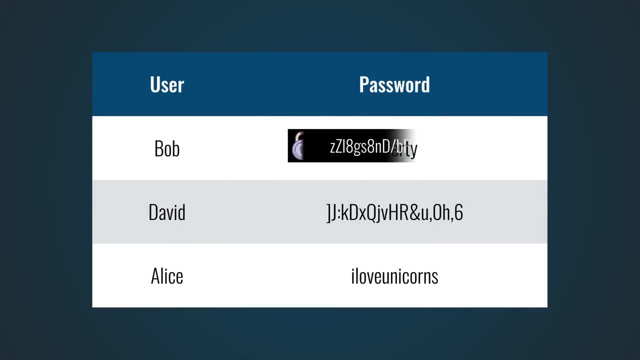 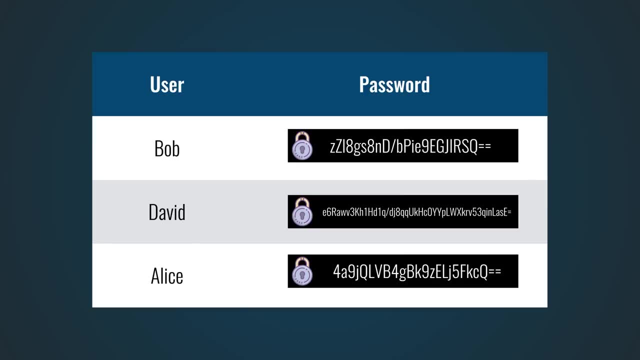 take the password of the user and, before you store them, encrypt them with an encryption key. This would prevent hackers from obtaining the real password of users, but it's still quite risky. Underneath the encryption layer is still a plain text password, And so 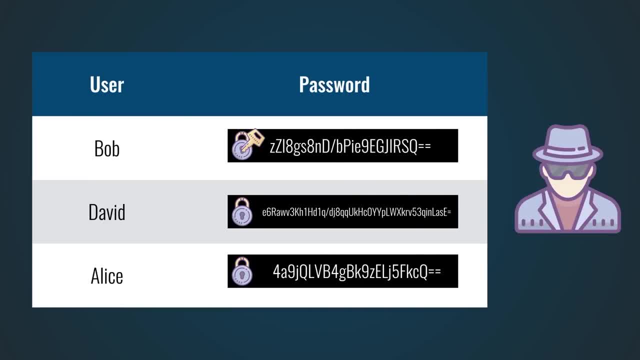 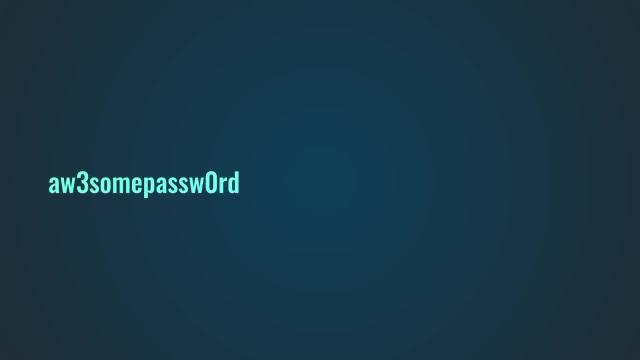 if an attacker manages to steal the encryption key as well, he can unlock all the passwords. The problem with encryption is that it is designed to work in two ways. You can encrypt the user's password to keep it safe, but you can also decrypt it to reveal the password again. 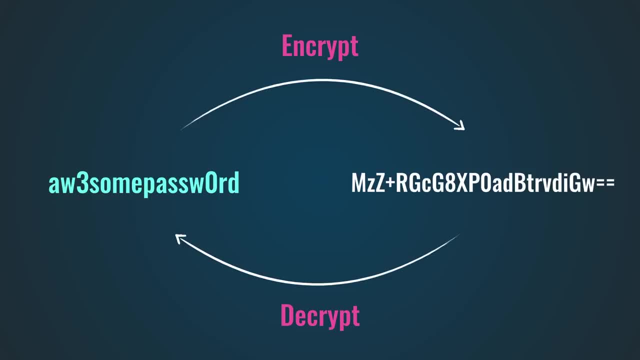 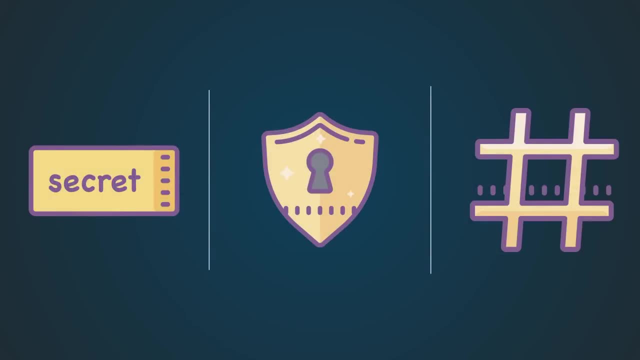 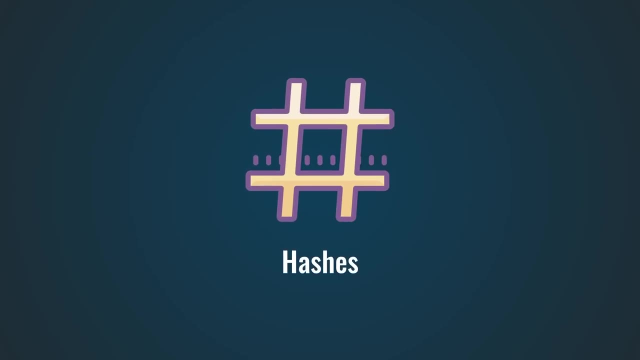 Encryption is very practical when you want to share data in a secure way, but not great if you want to prevent hackers from breaching your password. And that brings us to the third technique of storing passwords, and that's by using a hash function. How does that work? Well, a hash function takes an input. that could be a piece. 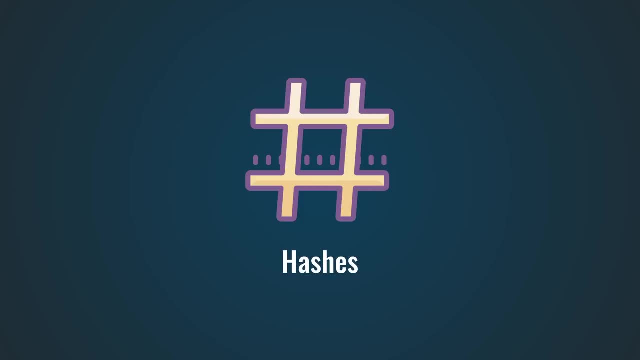 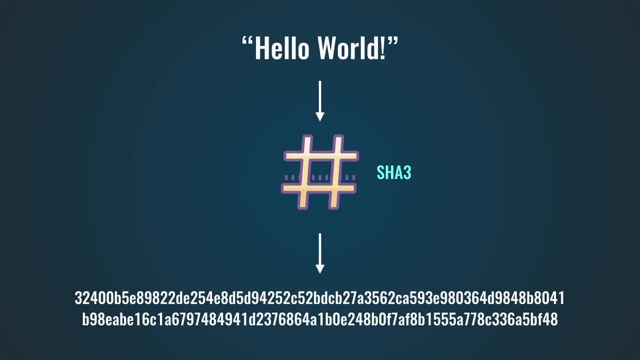 of text, like your password, or it could be a file, and it turns that into a string of text that always has the same length. There are many different hash functions available, but this is what the SHA-3 hash of Hello World looks like. Hash functions are very different from encryption. 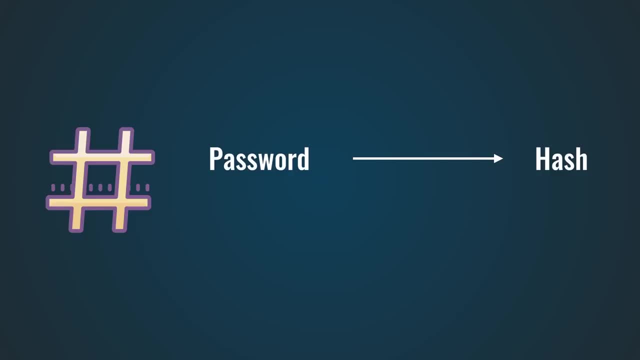 because they only work in one way. You can calculate the hash of a password, but you cannot take a hash and turn it back into the original data, And that is an interesting property to have. By using hashes, companies can verify that you're logging in with the correct password. 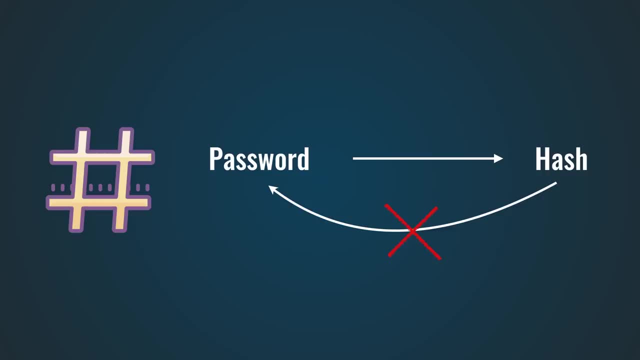 without having to store your actual password. However, they aren't perfect either. Most hashing algorithms are optimized for security. However, they are not perfect either. Most hashing algorithms are optimized for security. However, they are not perfect either. Most hashing algorithms are optimized for security. 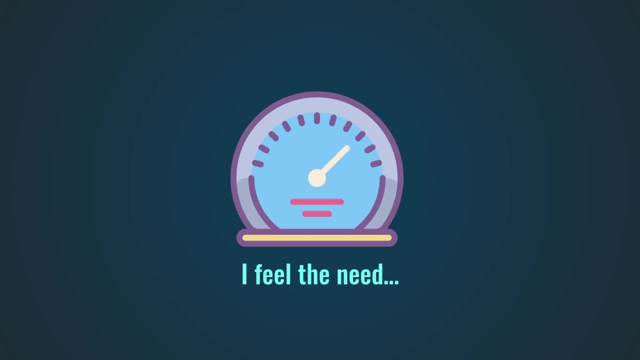 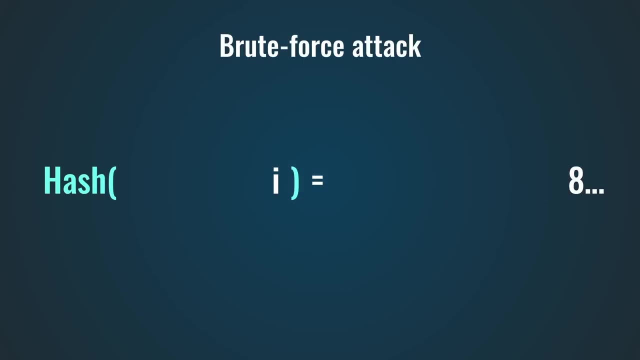 The more speed, the more hashes per second they can calculate, the better, And that makes them vulnerable against brute force attacks. By simply calculating every hash of every possible password, an attacker can reverse the hash function. A modern GPU can do this with a speed. 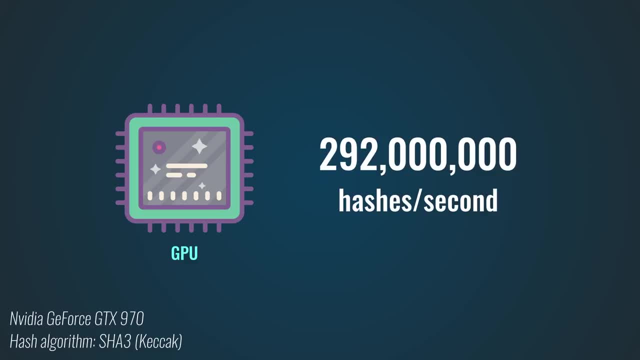 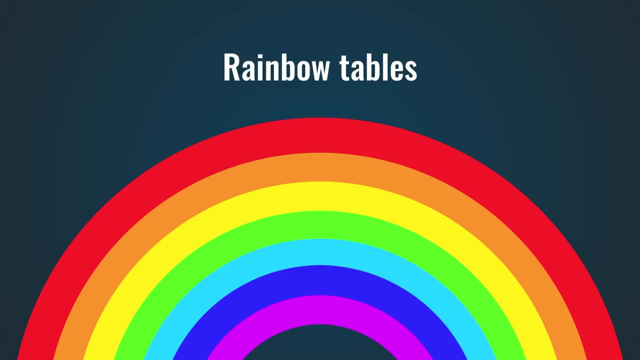 of 292 million hashes per second, so it's only a matter of time before a hashed password is cracked using this technique. And if that's not fast enough, hackers can also use rainbow tables to further accelerate the process. These are lists of pre-computed hashes that can be used to quickly. 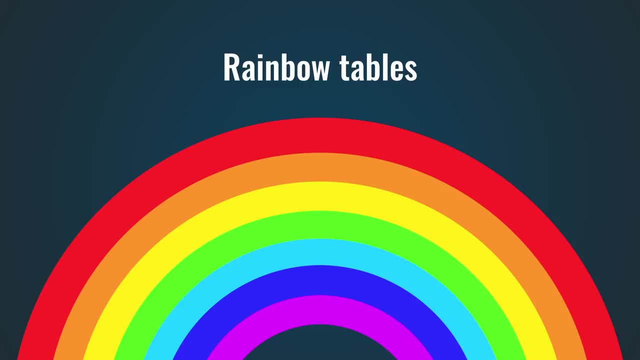 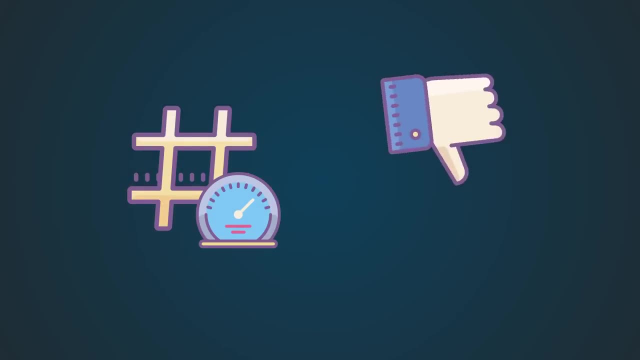 find weak and commonly used passwords. The speed of a hash function is a positive thing in certain areas. However, when it comes to storing passwords, you don't want this property. And then there is a second problem, And that happens when users share the same password, If 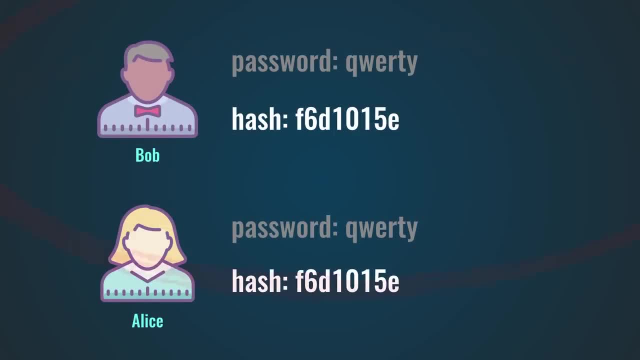 both Alice and Bob have the password QWERTY. the hashes of their passwords will be identical. So when a hacker cracks the password, the hash function will be the same as the hash function. So when a hacker cracks the password, the hash function will be the same as the hash function. 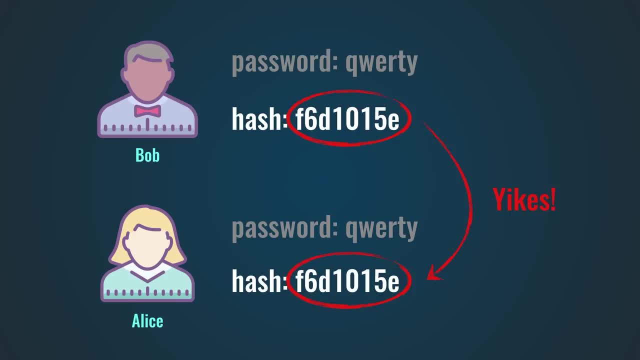 So when a hacker cracks the hash of this password, he also knows the other. Now you might think that's not a big deal, because it's very unlikely that different people will use the same password. Well, think again. The password QWERTY has been found more than 3. 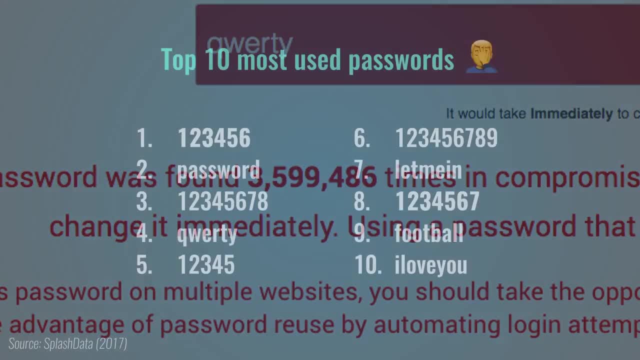 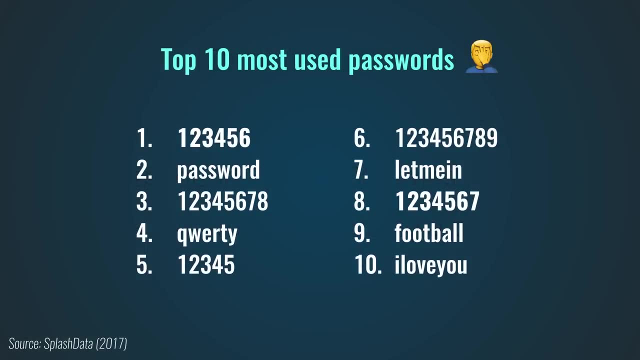 million times in data breaches. To make matters even worse, here's the top 10 most used passwords in 2017.. Not the strongest of passwords. To defend against these types of attacks, we can add what's called a salt to the password before we hash it. 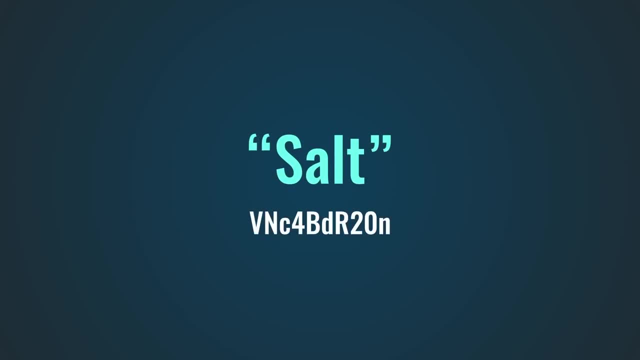 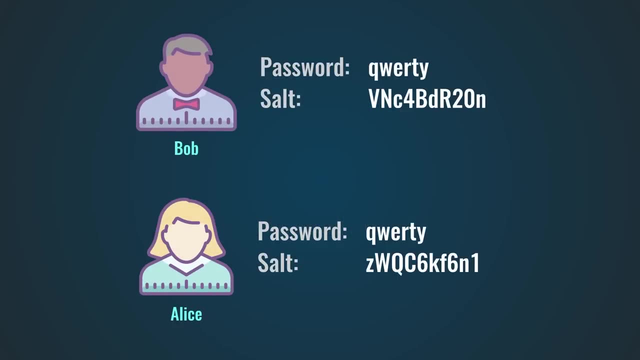 The salt is just some random data, but it ensures that the hash of your password will always be unique, even if others use the same password. So if Bob and Alice both use the password QWERTY, their hashes will be completely different. So if an attacker cracks Bob's password, he can't link that password to Alice and he has to start his cracking attempts all over again. This technique prevents hackers from cracking a bunch of passwords in one go. It makes a brute force attack slower, but still very much possible. 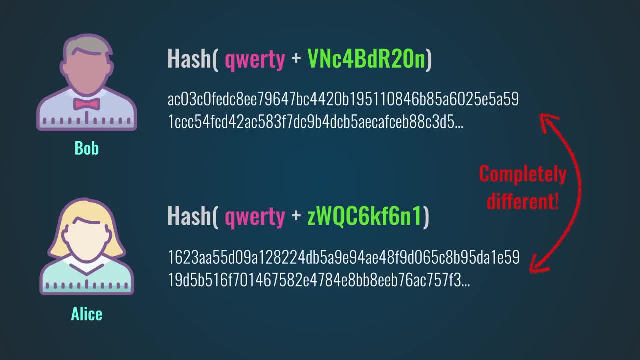 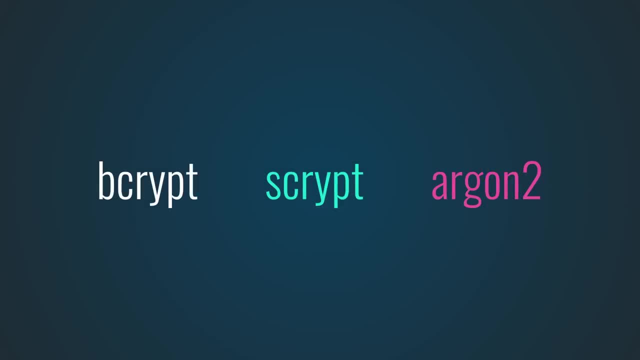 So to solve this, we have to take a look at another technique, which is using a special hash function which is deliberately being slowed down. Example of these are bcrypt, scrypt or argon2, and they completely neutralize brute force attacks. 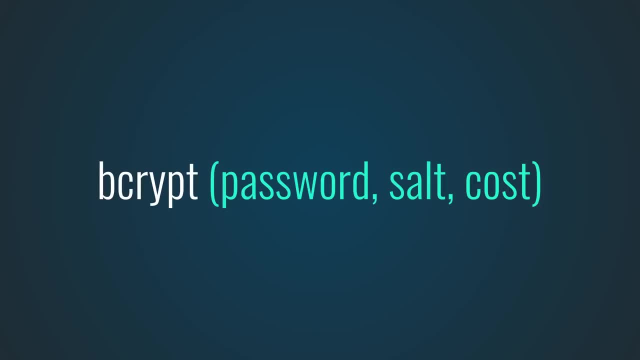 These algorithms take a password as input, along with a salt and a cost. This last one is very interesting. The cost defines the number of rounds the algorithm goes through and this affects the number of rounds the algorithm goes through and this affects the number of rounds. the 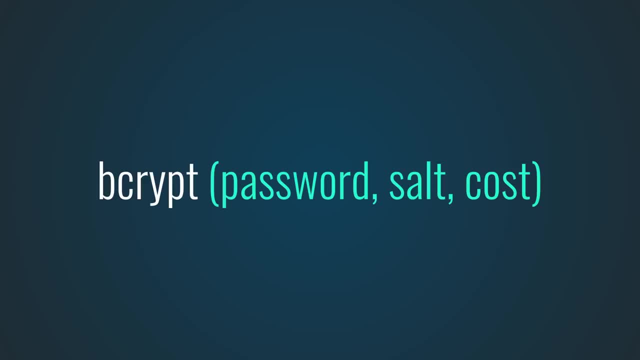 algorithm goes through, and this affects the number of rounds the algorithm goes through, and this effectively slows it down. Over time, our computers become faster, and so brute force attacks against these algorithms become easier, And that's because they can simply try more combinations in a shorter time span. 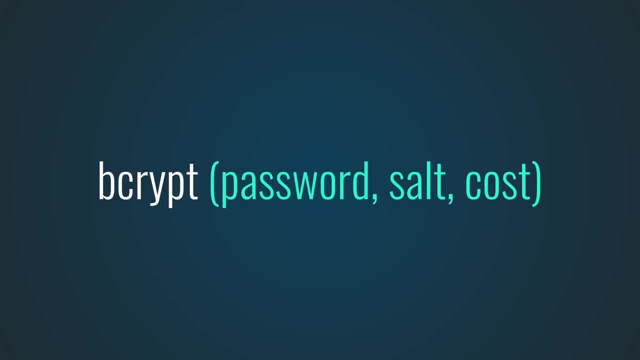 All we have to do to counter this is increase the cost parameter, so the algorithm remains resistant against these types of attacks. Pretty genius. So those are the three options that a company has to store and protect your passwords. But why settle for just one method if we can use more? Multiple. You can't be greedy enough when it comes to security. This multi-layer protection is used by Dropbox, for instance. They take your password and start by running it through a simple hash function without a salt. This is their first line of.